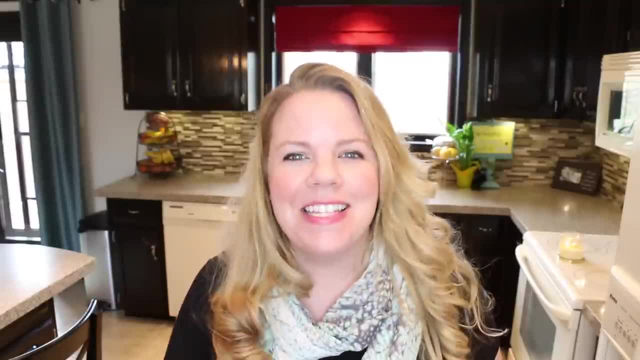 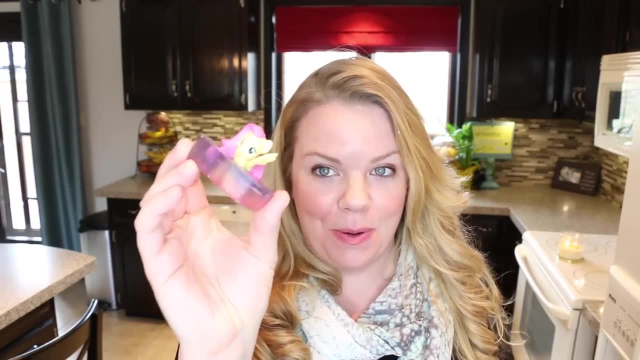 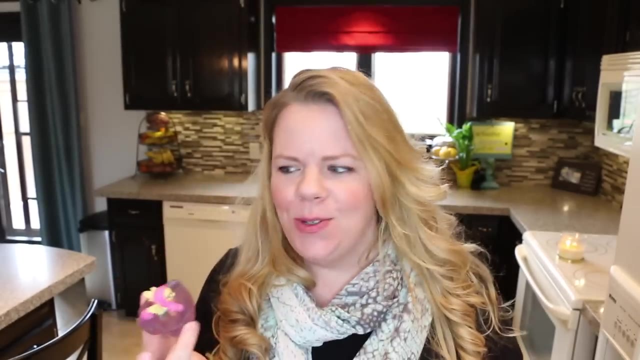 20 seconds, A 20 second craft. It's really inexpensive and super fun And it is drum roll please, These adorable little soaps. So it's a soap with a toy in it. If you don't have kids, you don't have to put the toy in it, But if you do have kids and your kids. 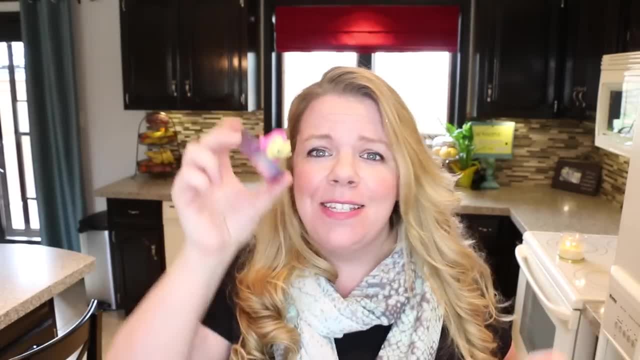 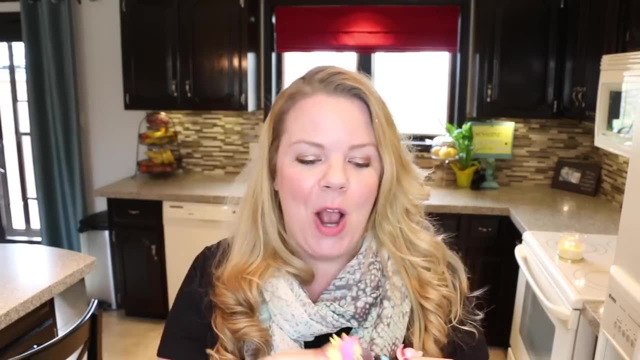 are like my kids, who like have an aversion to washing their hands Simply by putting a toy in their soap. They like want to wash their hands because it gets them to the toy faster. All you need for this is glycerin soap that's meltable, So you can. 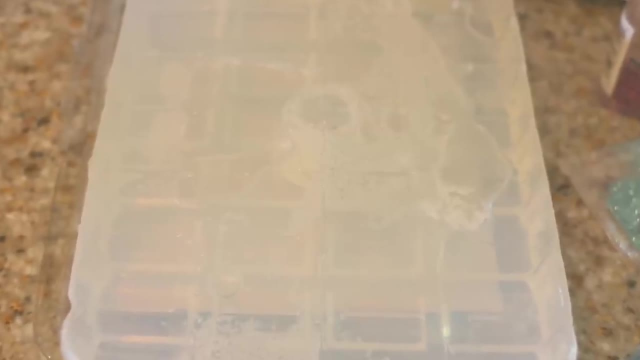 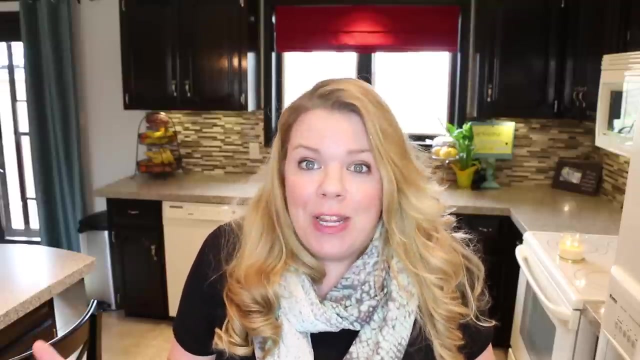 buy the blocks Really inexpensive. I got this entire brick. I bought it from Amazon- I'll put the link below- for about $9 and it made about 30 little bars of soap, So a really good price. We ended up putting some essential oils in it. The kids got to pick their own. 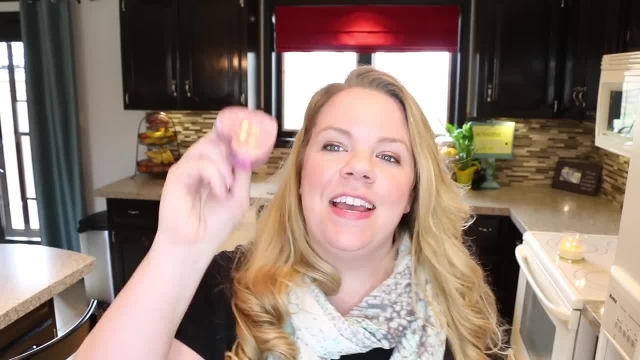 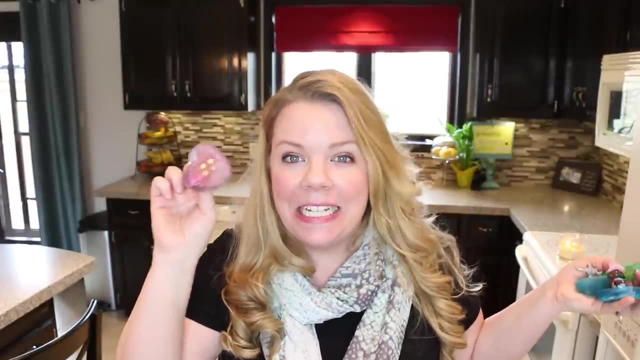 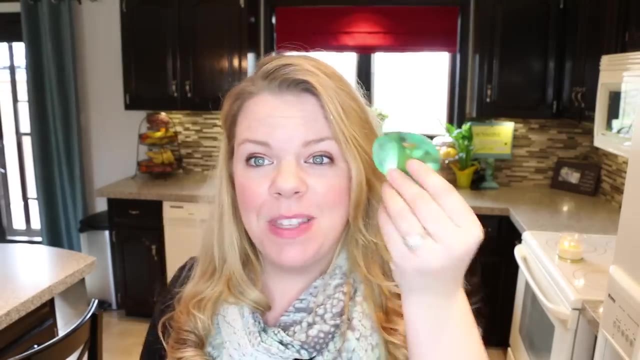 smells, but you totally don't have to do that. And we added sparkles. Can you see that? To get their hands sparkly clean, Get it Sparkles sparkly clean. So there's so many different fun things you can do. The toys are from the dollar store, So I got a pack of dinosaurs. 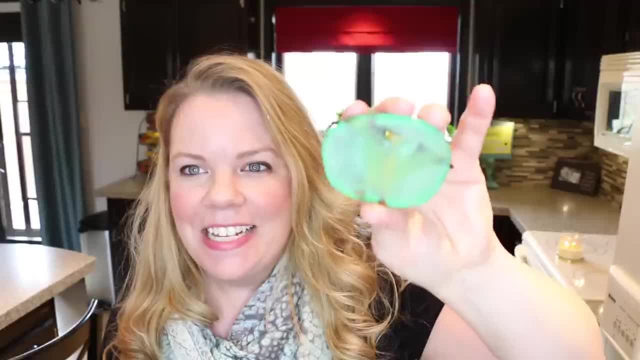 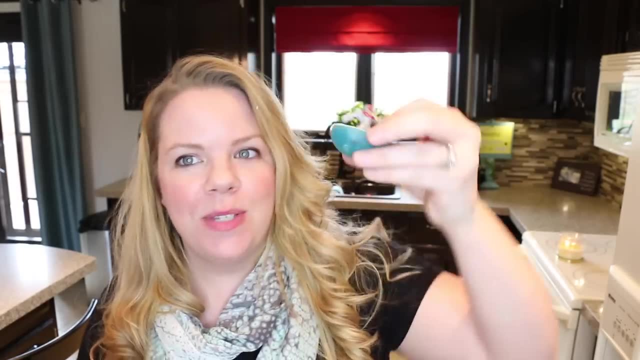 and I used an Easter egg- just half an Easter egg- to make a little pterodactyl like a dinosaur egg one. I got some little superhero toys from the dollar store and used again a half an Easter egg, sticking it out like this. The reason we ended up doing the toys like this, so they're. 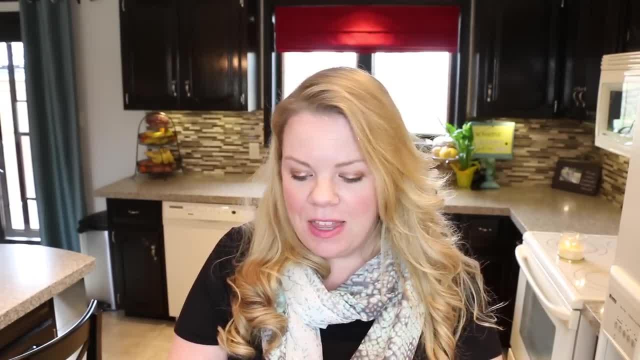 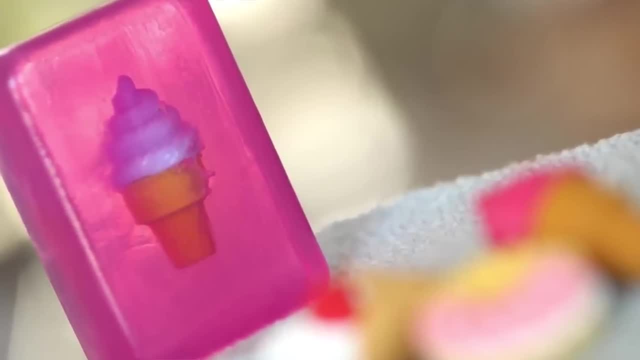 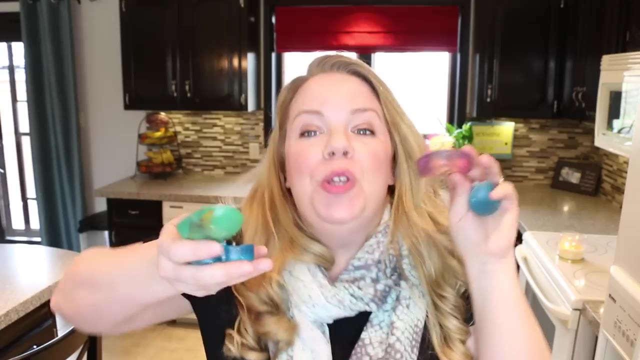 sticking out is because my sister-in-law said she saw these type of soaps at a boutique where she lives: $6 and it didn't even have color or sparkles, It just had like a dollar store toy in soap and they were flying off the shelves. You can make your kids a super. 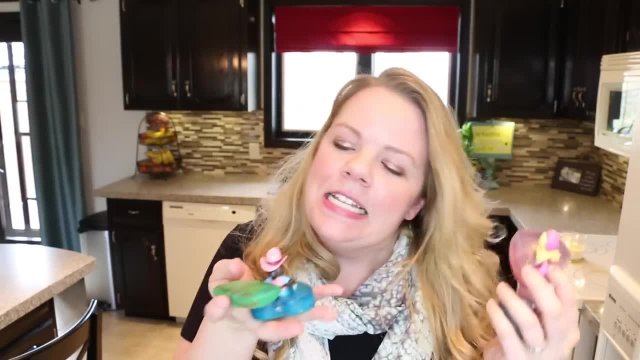 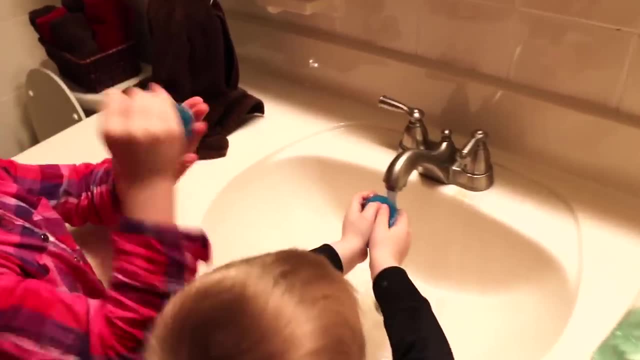 special little soap for them, With a toy in it. It's like a kinder egg, only you wash your hands with it, And it'll really encourage your kids to wash their hands. I'm going to show you how you can make these soaps so, so easy right now. So all you're 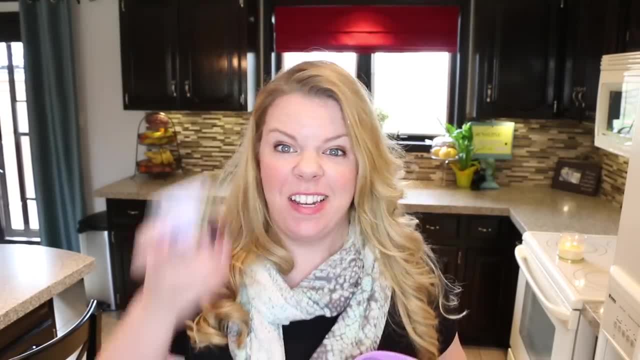 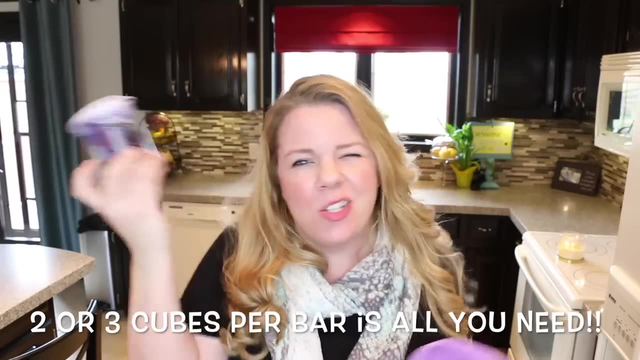 going to need is some glycerin soap and you're going to want to melt it in the microwave. I just use a cup. I wouldn't suggest using a styrofoam cup. I use this like cardboardy, or a plastic solo cup to melt it. 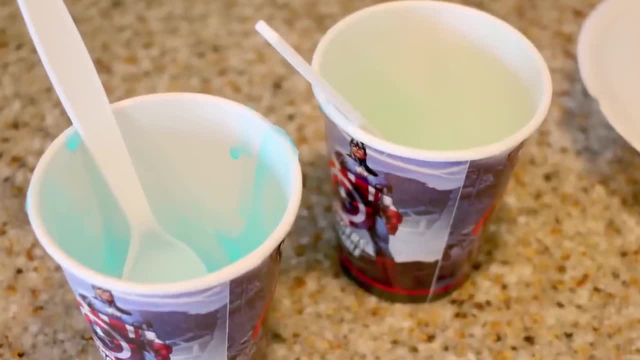 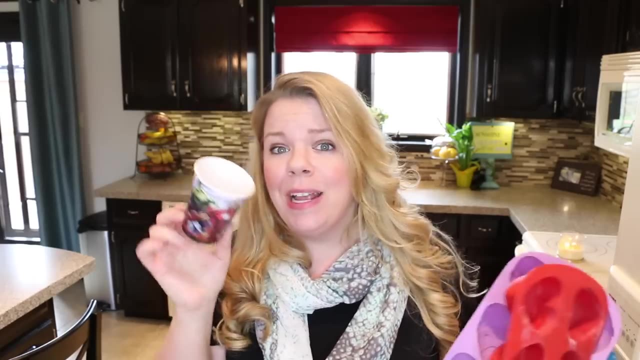 You only need to put it in the microwave for about 20 seconds- 20 seconds tops- to melt it. Then what you want to do is add either a scent or some sprinkles or some coloring, or you don't have to add anything at all. Next, you want to pour it. 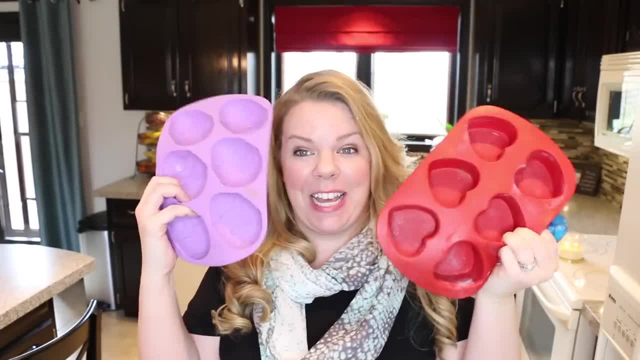 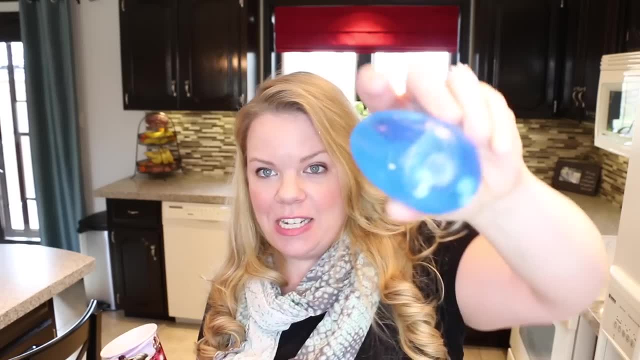 in a mold. You don't have to use a mold like this, Even the bottom of a cup. you can leave it in there and that'll work as a mold. Or you can use an Easter egg. Here is an Easter egg. We put half in the Easter egg at the top, let it cool, flipped it over, put the. 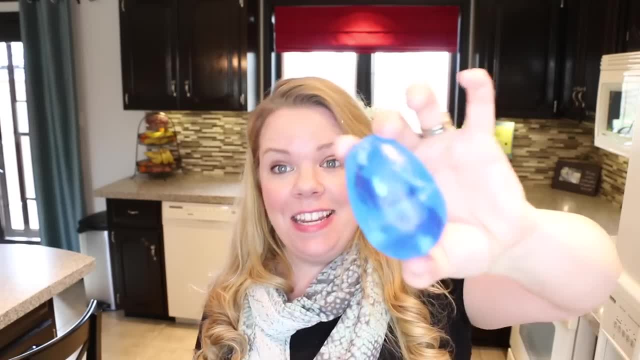 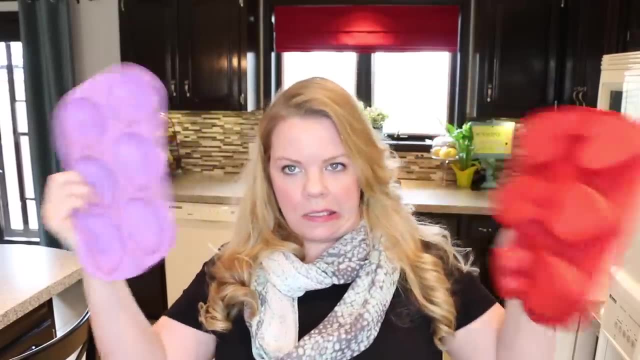 other half in And then squish the egg together to make an Easter egg soap. Or you can use these, you know, if you have any of these, you can even pick these up, sometimes at the dollar store, these jelly type molds. So we use the egg ones for the dinosaur eggs and the heart ones 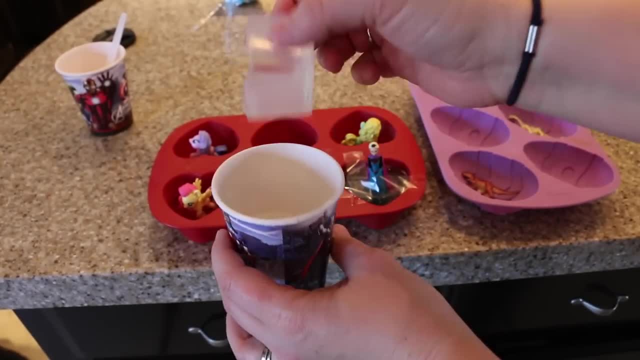 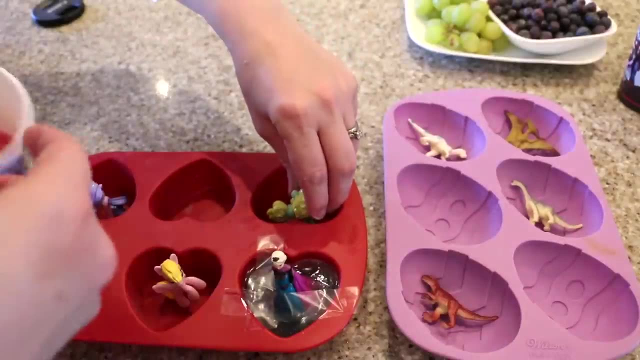 for the other ones. All you have to do is, once you've melted it, you can add color or sparkles or scents or nothing, and then pour it into the mold. You can use just about anything as a mold. Then you want to set in your toy. You can have the toy. 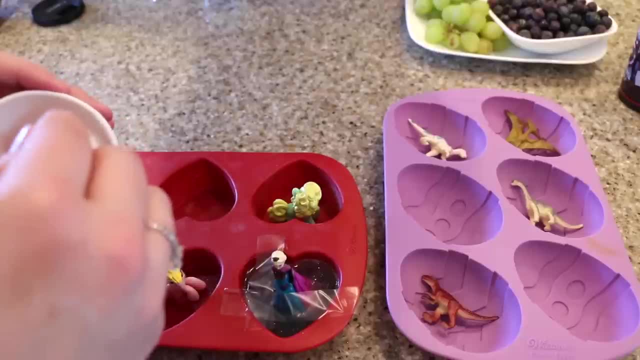 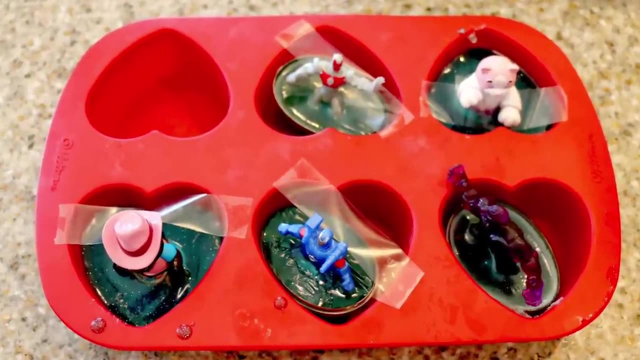 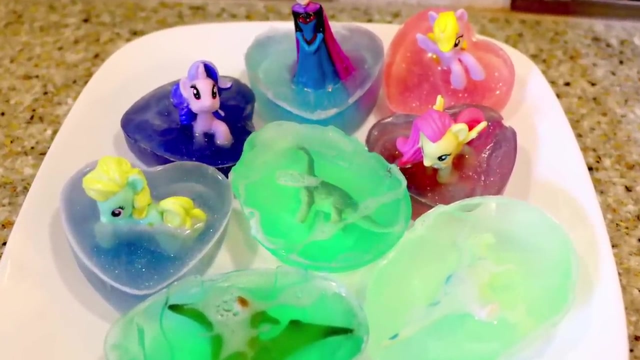 totally merged in the liquid soap or sticking up, like we have. If it's falling over, use a piece of tape to secure it up. Now, just simply let it harden for an hour and, voila, You have the coolest, coolest soap for your kids. 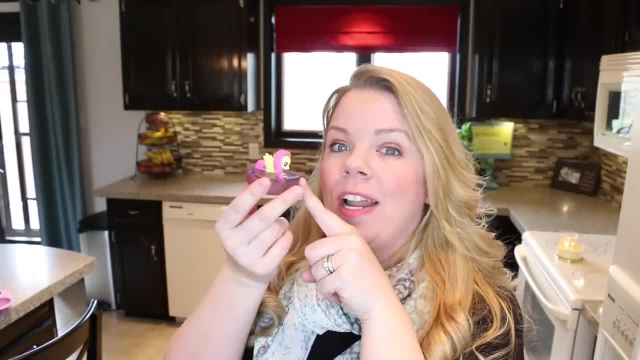 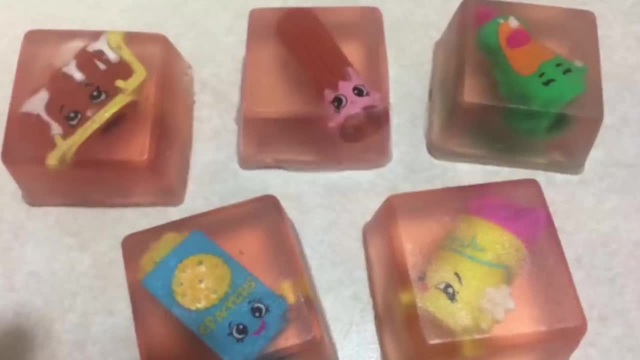 So that's it. you guys Melt some in the microwave, pour it into a mold, stick a toy on top. How adorable, It makes a really cute gift. If your kids are into Shopkins, how perfect would it be to put a little Shopkins in here. And the soap melts in about a week if they wash. 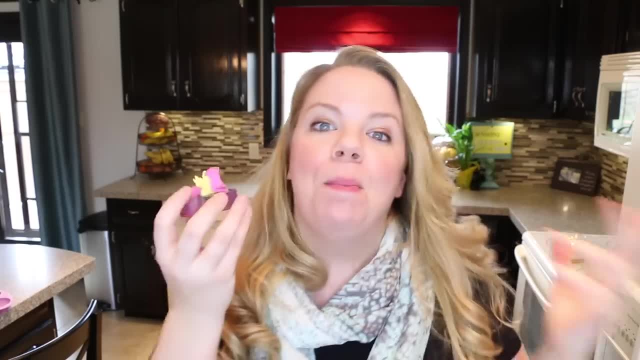 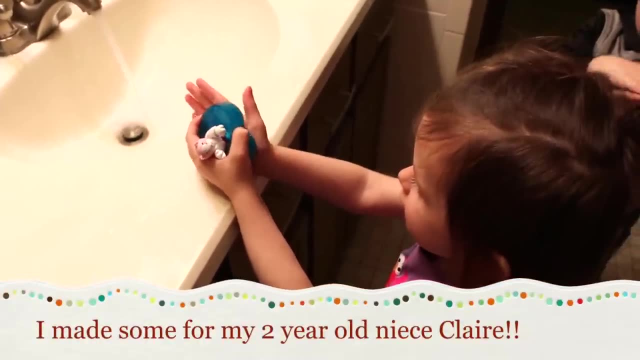 their hands multiple times a day and then they'll have the toy. My kids love to like play with their toys in the bath while they're like washing themselves. It's perfect, And with each bar being really inexpensive, it's a really fun bath toy that also does double. 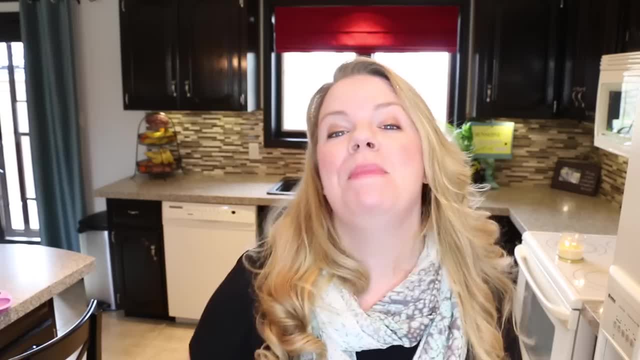 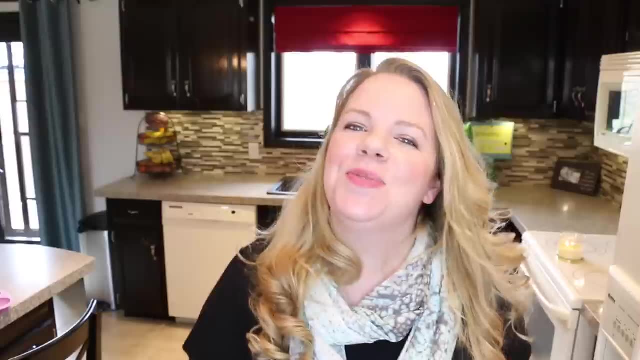 duty getting them clean. So thanks, so much. That's your tip. Make some soap today. I'm going to put the link below for the soap that I purchased Amazon, if you want to give it a try, and we'll see you next time. See you later.